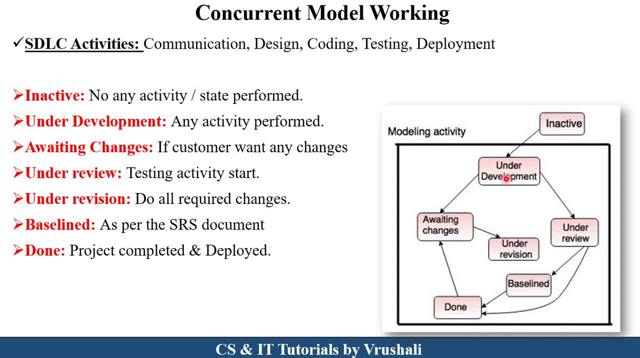 Then it move to next one, that is under development state. Under development state means first, that is communication. So first communication is performed here, that is, to collect requirement from the customer and plan accordingly. After communication they perform the design, here To design the product. and after design the coding perform here. So communication, design and coding, This state perform concurrently in under development state. 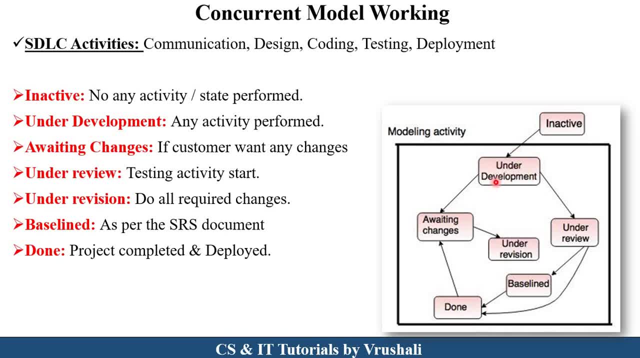 After that if customer want any changes in it it goes to awaiting changes. state Means customer want a particular changes So they collect requirement from the customer- new requirement and do all the necessary changes in under revision state Okay. Awaiting changes means collect requirement from the customer. Customer want a changes Under revision state means do all the required or necessary changes here. 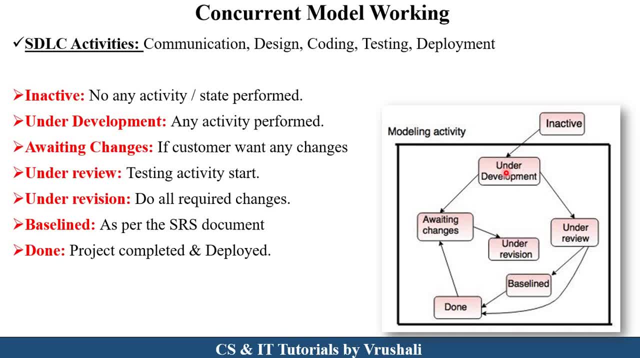 If customer didn't want any changes, Then this under development state directly go to under the review Means after communication, design and coding they goes to under the review. Under review means testing phase. Here tester test complete product and check that whether it is customer requirements match or not. 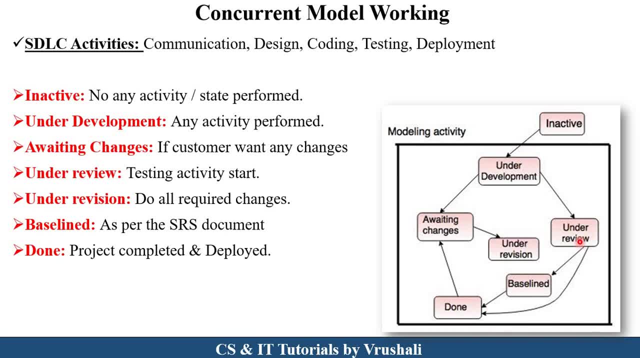 That is under review means testing phase. After under review, it move to next state. that is baseline Means it check that complete product is as per the SRS document or not. And after baseline And after baseline it move to done state. Done means your project is completed and deployed to the customer. 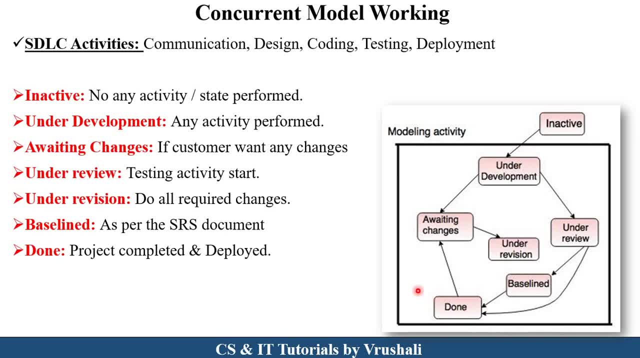 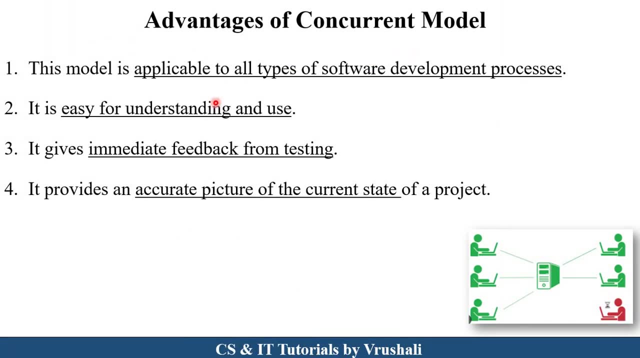 And after completing if customer want any changes, then it again go to awaiting changes. state in this way Clear. So basically, concurrent model display the state of each and every activities. Next Now the advantages of concurrent model. The important advantage is it applicable to all type of software development process. 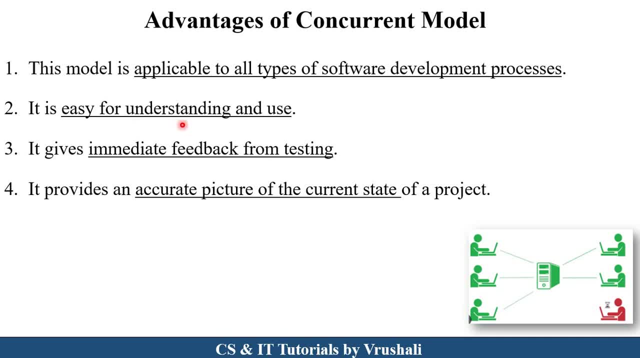 It is very easy to understanding and use Because it display state of each and every activities. It gives imaged feedback from testing. There is a special one state which customer collected their feedback. Now it provide the accurate picture of the current state of the project. 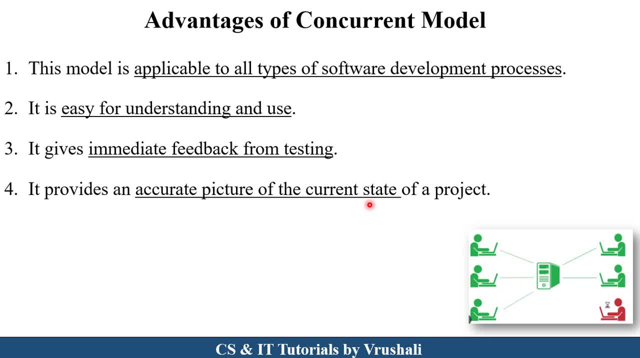 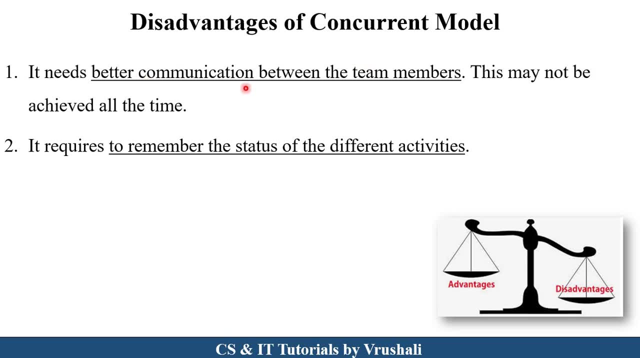 It display which activity have performed Right. Next Now the disadvantages of concurrent model is: There is a need for better communication between the team members, Because if customer want any changes, it moves to another state Right, So communication is must here.